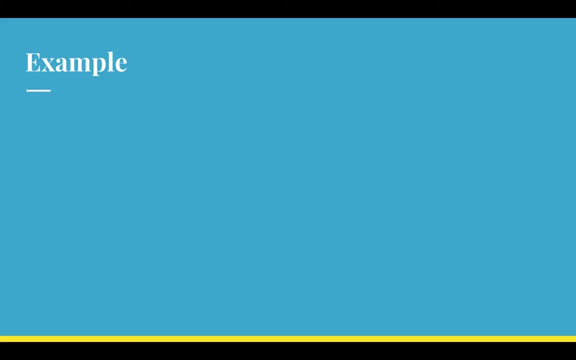 you solve. So let's look at a story problem. Here's an example. Ellie had nine books and Cole had five. How many more books does Ellie have than Cole? I always like to look at how many more books Ellie has than Cole. I always like to look at how many more books Ellie has than Cole. I always like to. 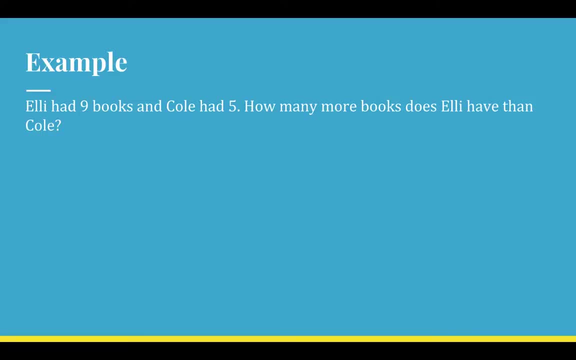 start by looking at the keywords and remember that was how many more or how many fewer. So I'm going to look for those two phrases and I see them right here. How many more books does Ellie have than Cole? So, by when I see that, how? 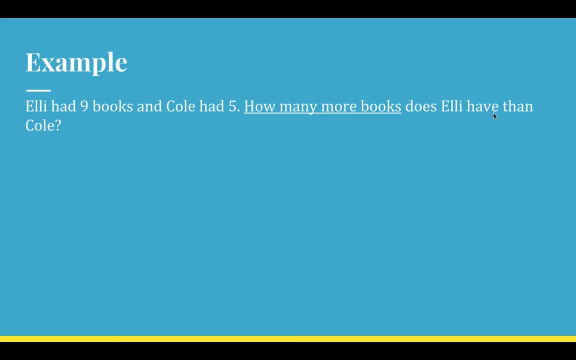 many more. I can tell that I will be comparing. Next, I like to look at the important numbers so I know what numbers I'm working with. I see that Ellie had nine books and Cole had five, So I'm going to circle those so I know that. 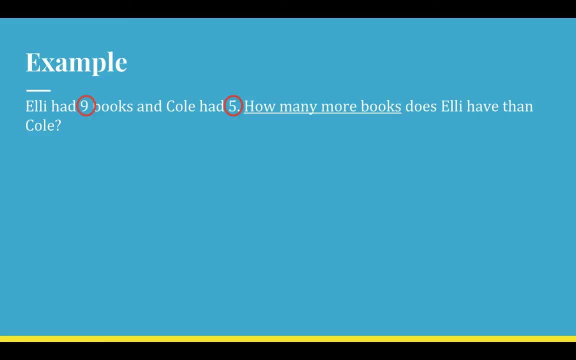 they are important. They're the numbers I'm focusing on. Next I can start doing a strategy to help myself. One of my favorites is drawing a picture, So I'm going to draw a picture to represent what the story problem says. I like to draw circles because they're quick, easy and I can see. 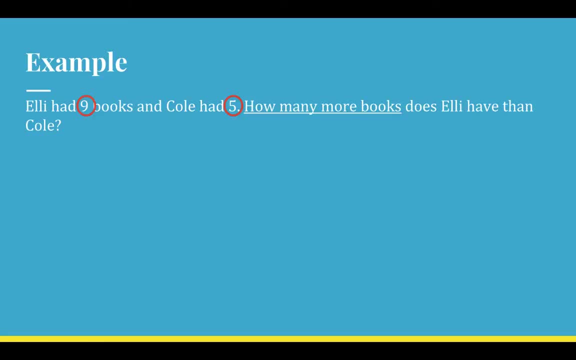 them very easily. So I'm going to draw circles with E's in the middle for Ellie and it says that Ellie had nine books, So I'm going to start with that. So Ellie had one, two, three, four, five, six, seven. 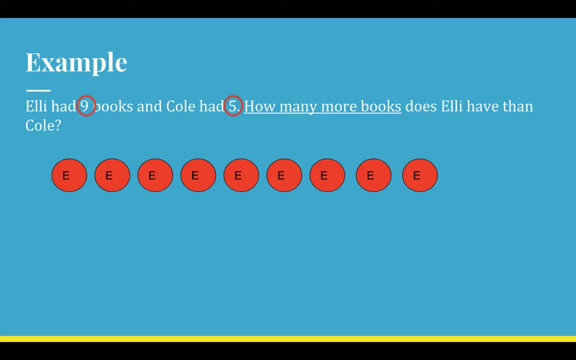 eight, nine. Those nine circles with E's represent the nine books that Ellie had. Next I'm going to draw how many Cole had and I'm going to draw them right underneath. So Cole had five, it says here in the story problem. So underneath. 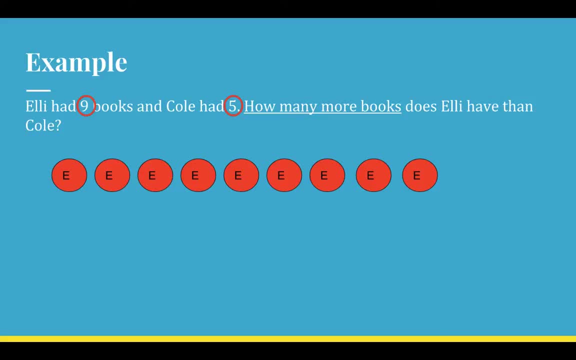 I'm going to draw circles with C's in them for Cole's books. So one, two, three, four, five, The letters on them just help me to keep them straight, as well as the colors, so that I can get them in there. And now I'm going to start with the. 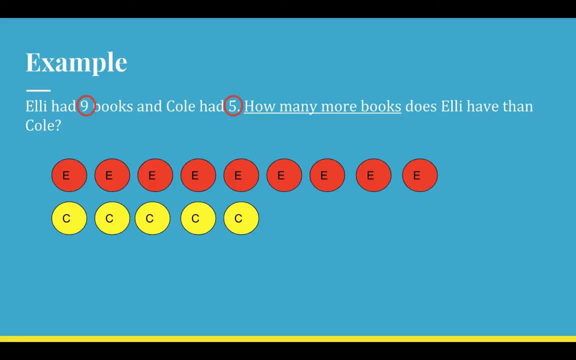 easily see the difference between the two. I don't always have colors to change, so writing the letters helps me keep track that the ones with E's are Ellie's and the ones with C's are Cole's. Next, as I'm comparing, I'm going to draw lines in: 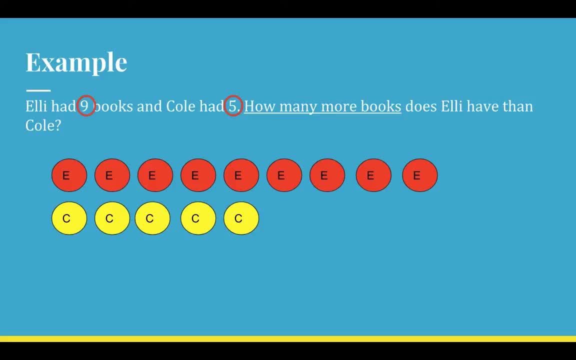 between the ones that have a buddy or that match up. So you'll see that when I drew my circles I lined them up nicely so that I don't have to cross over. So I'm gonna draw a line down to the ones that match like this. So I see these two. 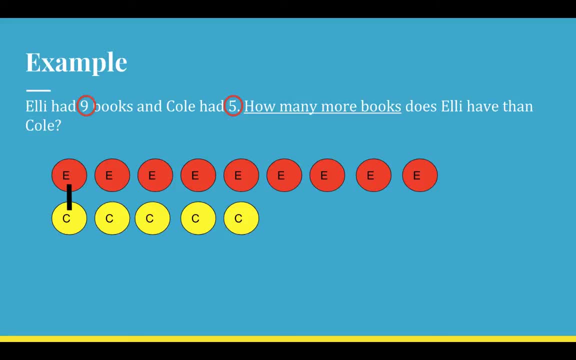 one from Ellie's and one from Cole's. They would match up to have a partner. I can see that those two match, They line up, These two have a match, These two have a match. And these ones- Now that I'm there, though, these extra ones off to the 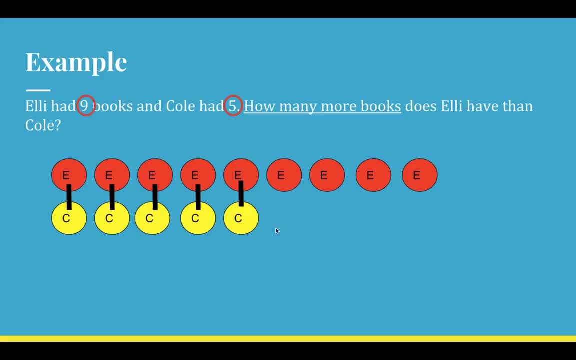 side there's no more books that can match up. Cole doesn't have any more, So these ones would be the extras that Ellie had more than Cole. So these extras over off to the side are how many books they have. So I'm going to draw a line. 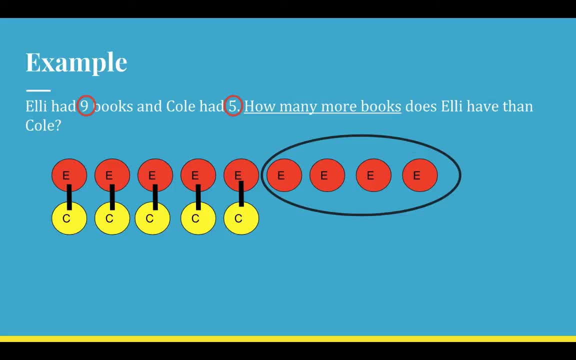 that shows how many more Ellie has than Cole. So I see that there are 4 circles, So I know that Ellie had 4 more books than Cole. Another way to look at this is: I can use subtraction. So when I'm using subtraction, I'm going to start with a bigger number. 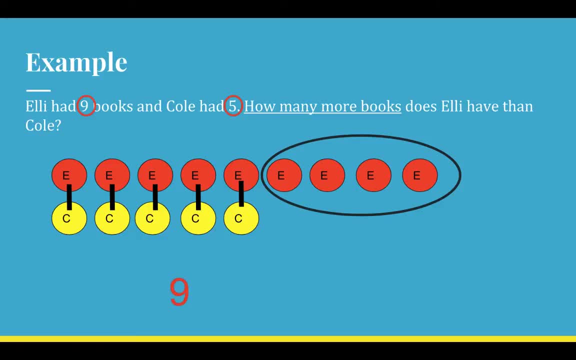 So that's what Ellie had, So I'm going to have 9.. Then, to figure out how many more I have to subtract how many Cole did have, because I'm at the difference between the two. So I'm going to subtract and I'm going to subtract five Those. 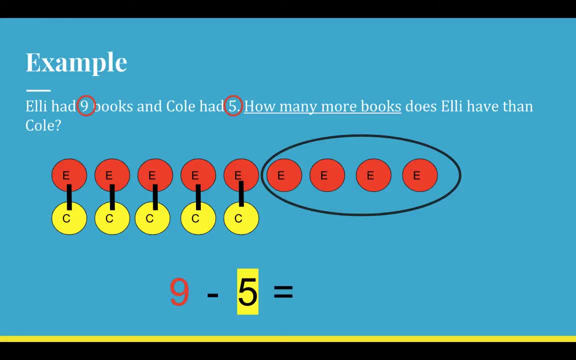 are the yellow ones, So nine minus five. I can look at this a couple of different ways. I can count backwards If I want to look at it at a part-part-whole box. I can use a part-part-whole box over here, Thinking back to our lesson before, where we know that nine would be the whole it's. 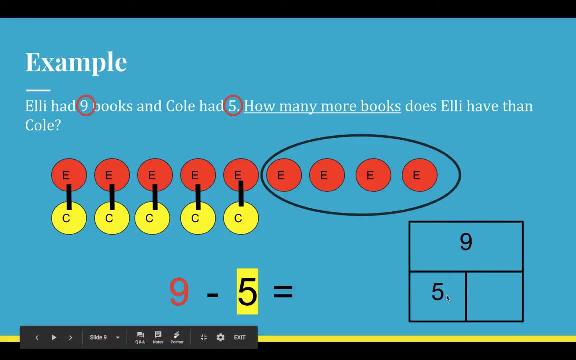 the biggest number, and five is the part that we know. That's how many books Cole has and we want to know how many more. That's the other part. So, as I use that part-part-whole box, I know that the 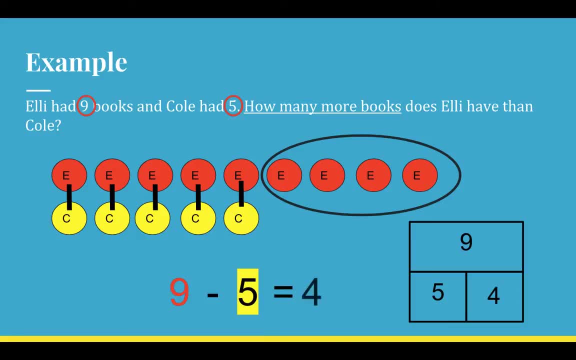 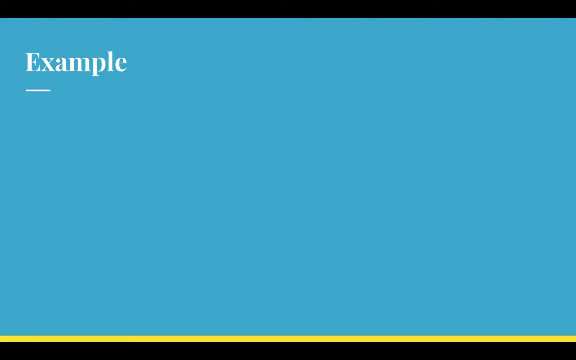 other part is four. I also know that nine minus five is four. So we have three different ways to show that Cole had four fewer, or Ellie had four more books than Cole. Let's take a look at another example. Kenley got ten pumpkins and Jamyla got four. How many more pumpkins did Kenley get than Jamyla At? 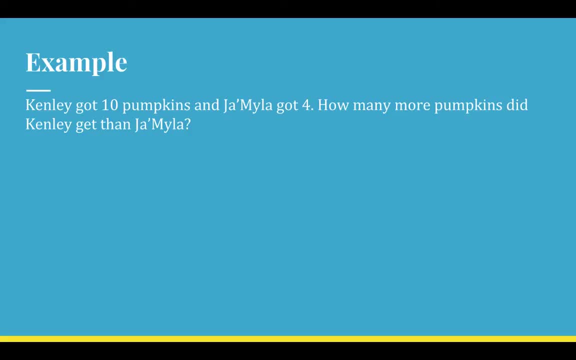 this point. you can pause and see if you can solve it on your own. Try drawing a picture using an equation or using a part-part-whole box. Did you give it a try? Let's try it together and see if your strategy matches mine. So let's look at the problem again. Kenley got ten pumpkins and Jamyla 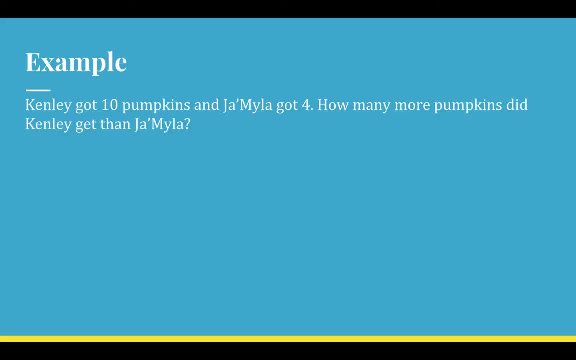 got four. How many more pumpkins did Jamyla get? Let's try it together and see if your strategy matches mine. I'm going to start by looking at those keywords. Which keywords are they? Yep, you've got it. How many more is the keywords to know? So we know it's going to be a comparing problem. Next, I'm 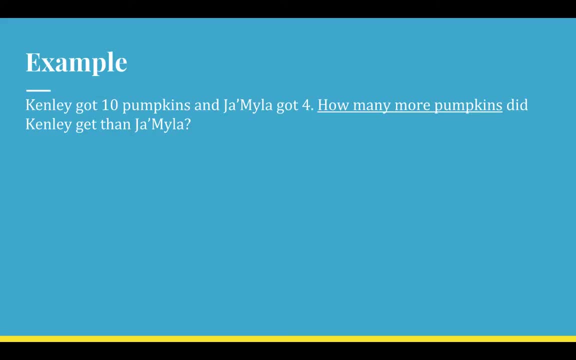 going to look at the numbers. Which numbers should I circle? You've got it. I need to circle four and ten. Those are two important numbers that I will need to know. Next, I'm going to draw a picture, So remember, I like to draw circles and to keep everybody's pumpkin straight, I'm going to use the. 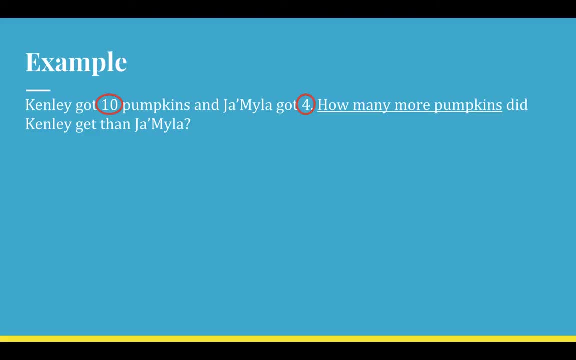 first letter of their name inside, because I don't always have colors and it kind of wastes some time if I'm going to color them in. So I just draw a circle with a letter in the middle and that helps me save time and I can still use my strategy. So Kenley had how many pumpkins? Ten, So I'm going to. 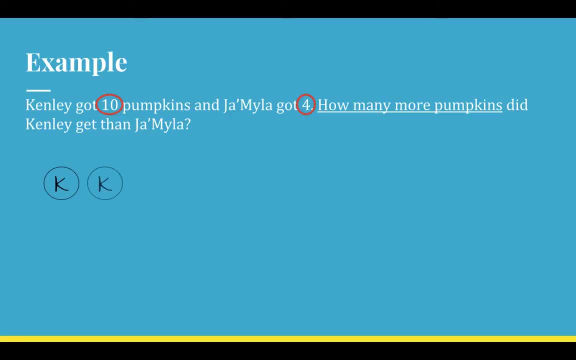 draw ten circles with K's in the middle: One, two, three, four, five, six, seven, eight, nine, ten. Those are Kenley's ten pumpkins. Next I need to think about how many Jamyla got. 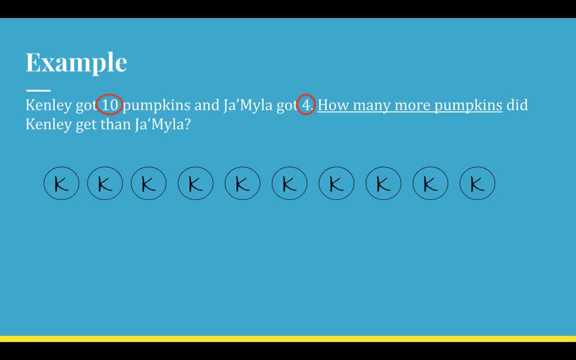 because I want to figure out how many more pumpkins Kenley got. So if I'm going to compare them, I need to see all of them out there. Jamyla got four, so I'm going to draw four circles with a J for Jamyla. 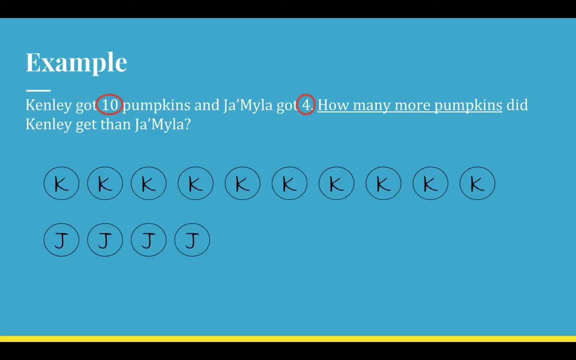 One, two, three, four. Now that we have everybody's pumpkins out there, if I'm comparing and drawing a line, I'm going to see which ones match up and have a buddy or a partner, The leftover ones that don't.